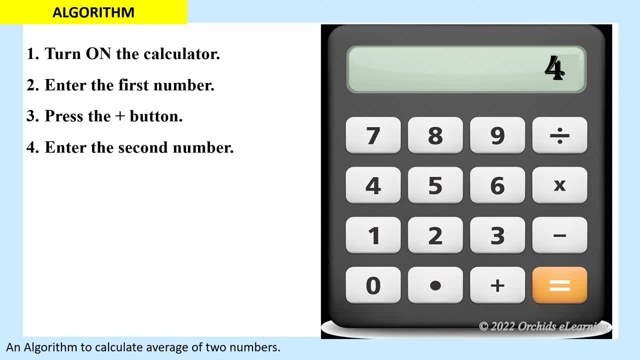 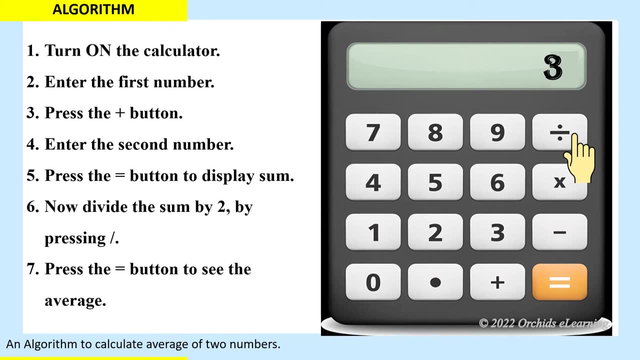 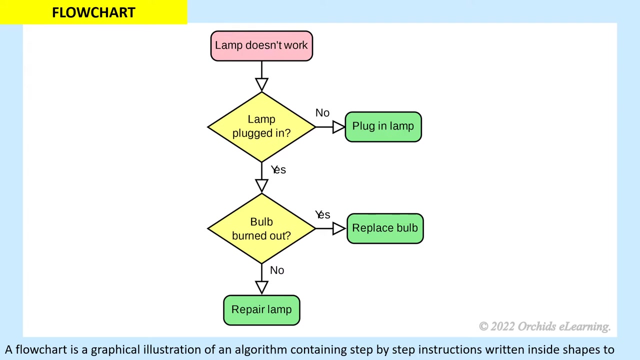 Enter the second number. Press the equals button to display sum. Now divide the sum by two by pressing backslash or divide button. Press the equals button to see the average. A flowchart is a graphical illustration of an algorithm containing step-by-step instructions, written in side shapes, to solve any problem. 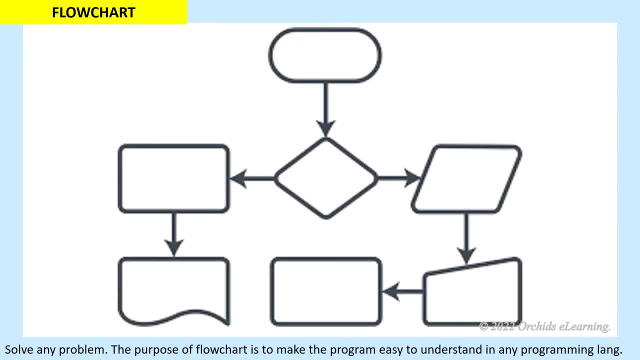 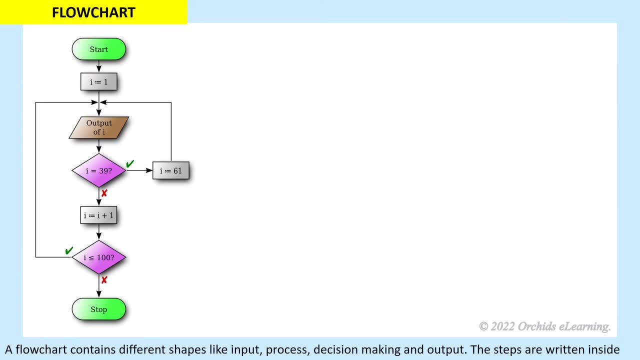 The purpose of a flowchart is to make the program easy to understand in any programming language. A flowchart contains different shapes like input, process, decision making and output. The steps are written inside geometric symbols and are connected each other through flow lines. 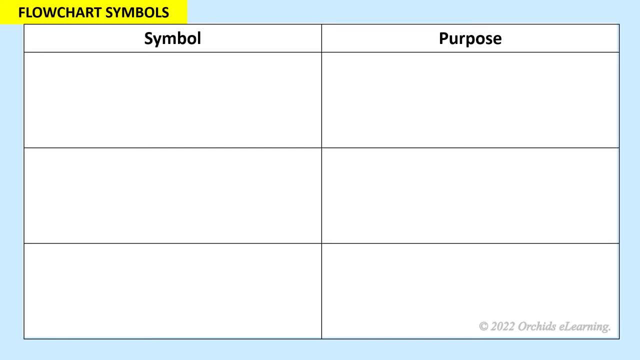 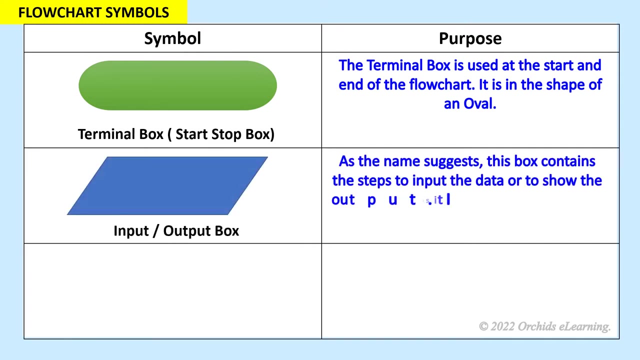 Let us see the different flowchart symbols. The terminal box is used at the start and end of the flowchart. It is in the shape of an oval. The input or output box contains the steps to input the data or to show the output. 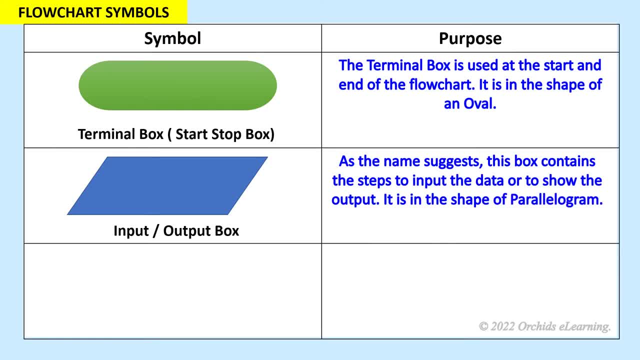 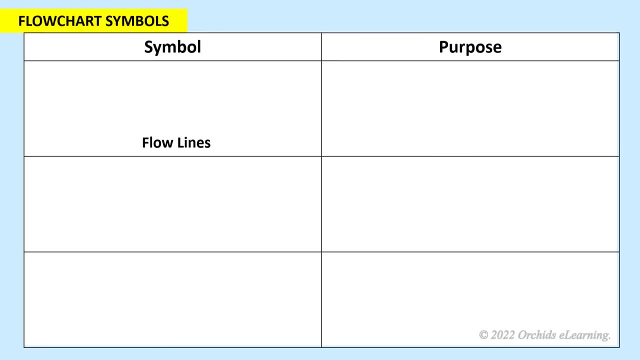 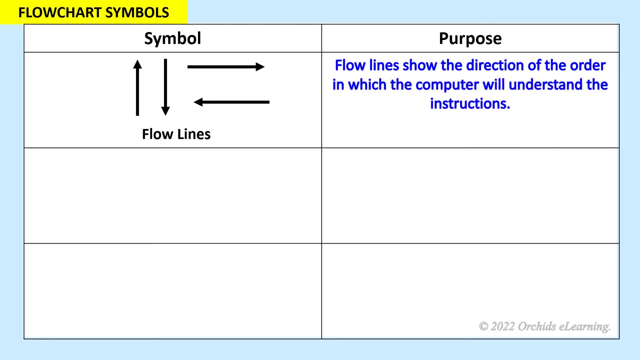 It is in the shape of parallelogram. The processing box is where all the processing steps are shown. Processing means calculation, data interpretation, etc. Flow lines show the direction of the order in which the computer will understand the instructions. The decision box demonstrates an operation that needs logical decision making. 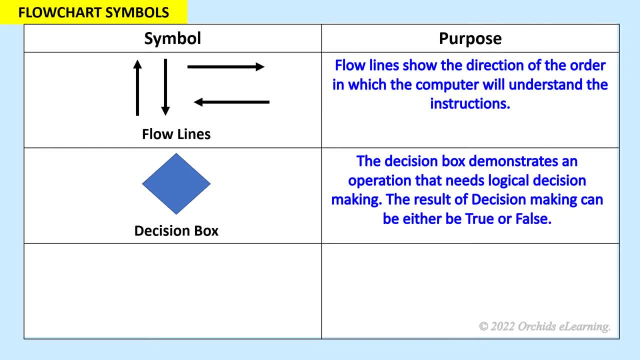 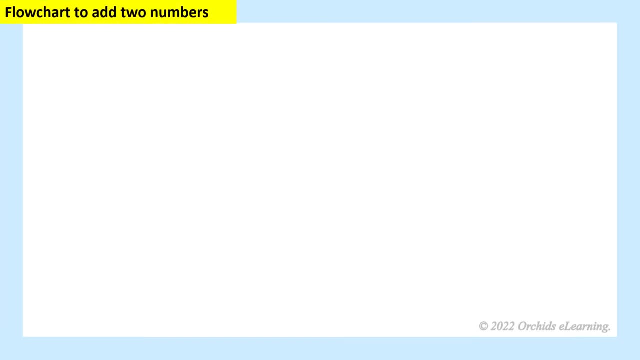 The result of decision making can be either true or false. The round shape connector is used when the flowchart is too long to fit on a single page. It connects the part of a flowchart Flowchart to add two numbers. The oval shaped terminal box marks the start of the flowchart. 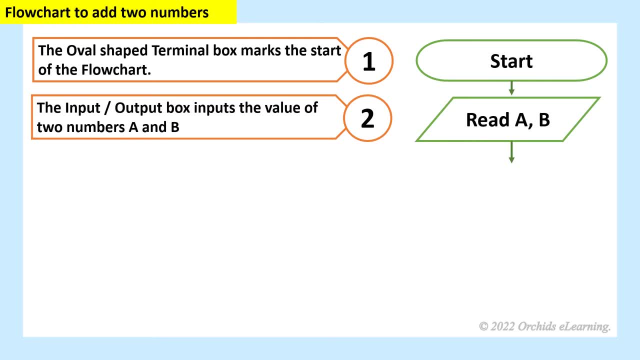 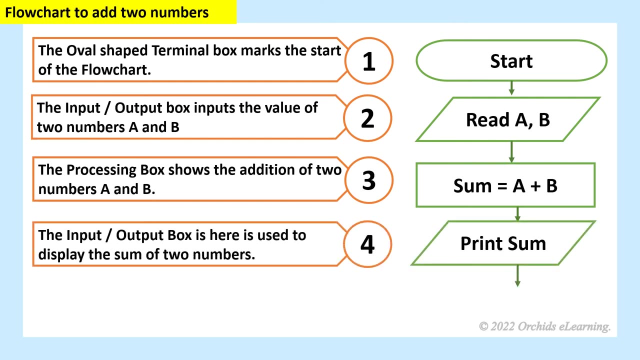 The input or output box inputs the value of two numbers, A and B. The processing box shows the addition of two numbers, A and B. The input or output box is here is used to display the sum of two numbers. The terminal box appears again.